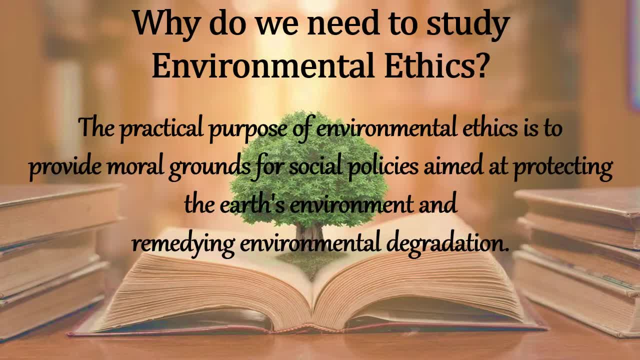 Environmental Ethics are a key feature of environmental studies that establishes a relationship between human and the Earth. With Environmental Ethics, you can ensure that you are doing your part to keep the environment safe and protected. This has degraded our planet's ability to provide the services we humans need. 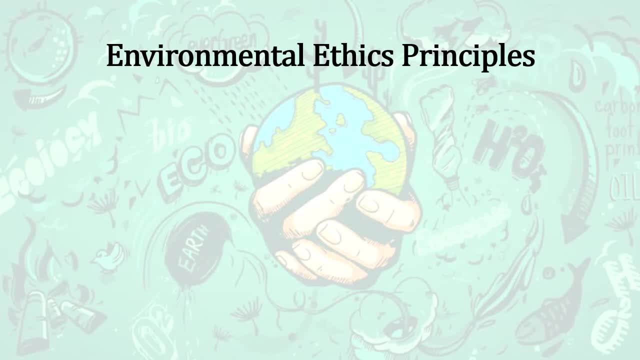 Environmental Ethics Principle. Here are some Environmental Ethics Principle. First, we should have profound respect for nature. People need to respect nature and living things because the environment is important. I know that hurting the environment hurts animals and pollutes the Earth when we don't. 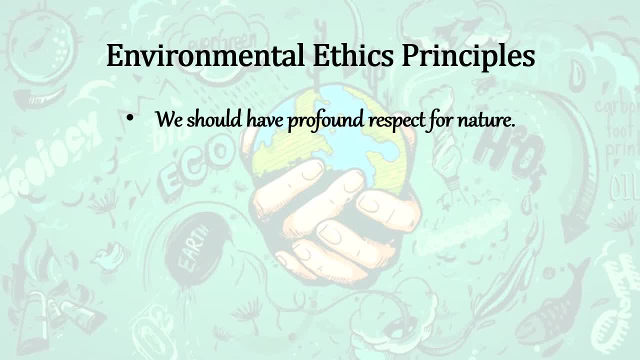 Without plants and trees, we will not be able to survive. The environment is also good and healthy for you and helps you breathe. Second, we must maintain our harmonious relation with our species. Psychological self-awareness helps us understand and accept ourselves and other people for what they are. 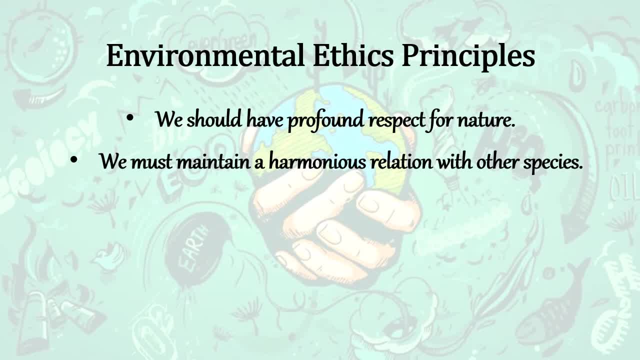 It makes us more tolerant and humble, But the ultimate spiritual method is based on freedom. Third, everyone should take responsibility for this impact of our nature, For pollution or global warming or for any such problem. people will blame the government and government will blame the people. 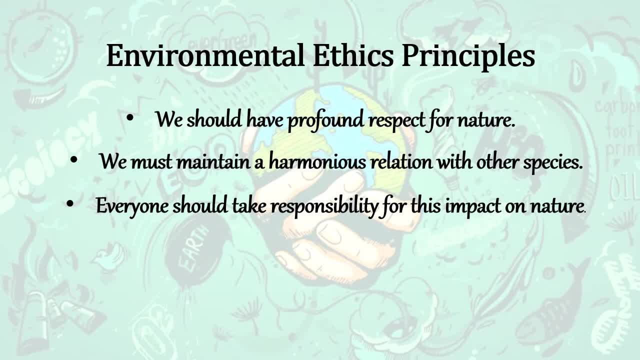 Who should actually take responsibility in solving such problems? That's why everyone should take the responsibility for this impact on nature. Fourth, local and indigenous environmental knowledge should be respected. And last, we must plan for the long term. When we say long term, 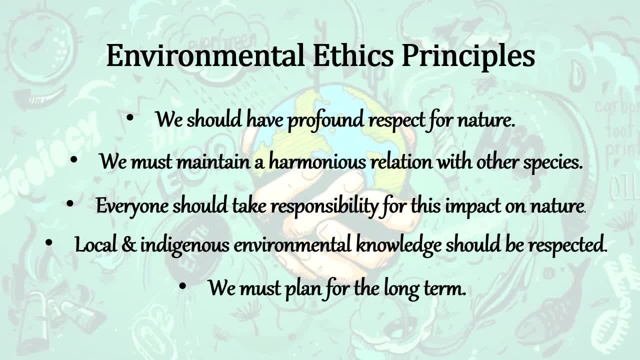 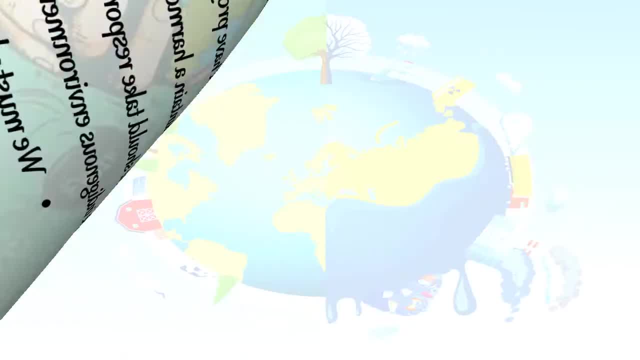 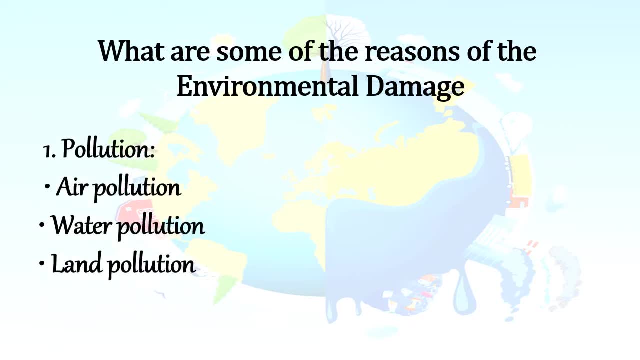 it includes overall goals for the company set for 4 or 5 years in the future and actually based on reaching the medium term. What are some of the reasons of the environmental damage? The first one is pollution, Three in one: Air, water and land pollution. 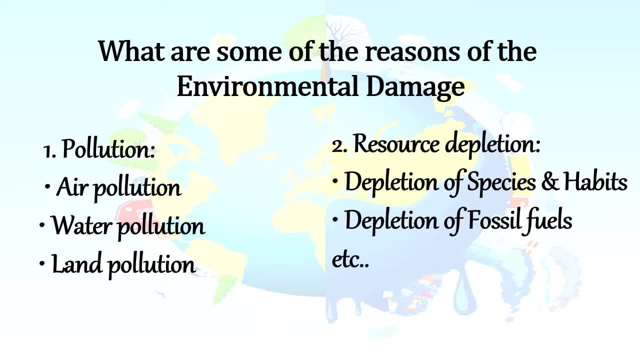 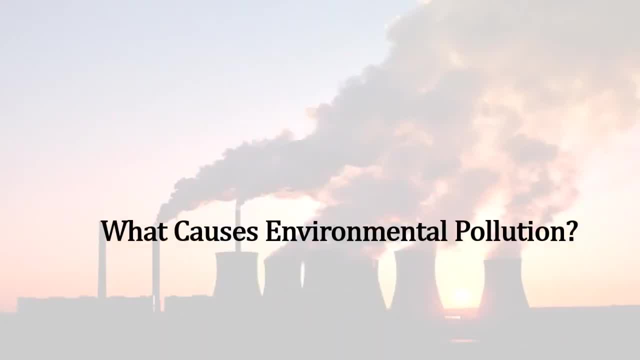 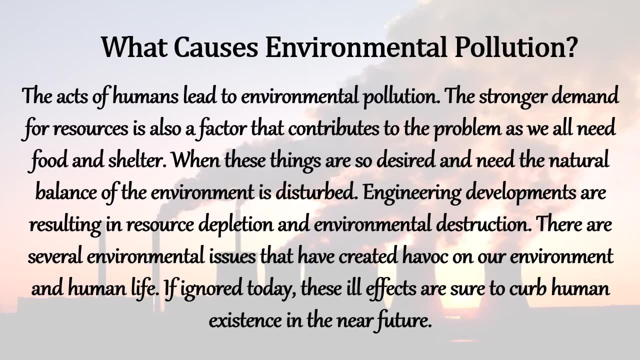 And the second is resource depletion: Reduction of species and habits, Reduction of fossil fuels And et cetera. What causes environmental pollution? The acts of humans leads to environmental pollution. The stronger demand of resources is also a factor that contributes to the problem. 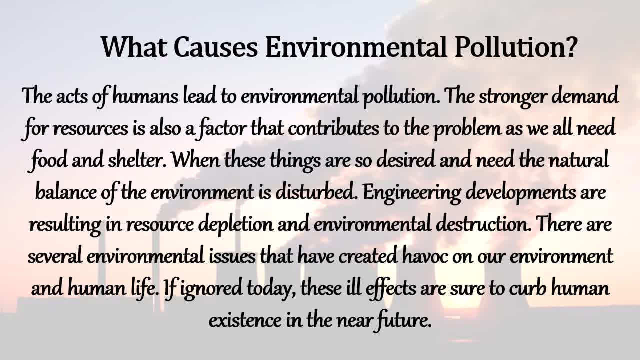 as we all need food and shelter When these things are so desired and need the natural balance. the environment is disturbed. Engineering developments are resulting in resource depletion and environmental destruction destruction. There are several environmental issues that have created havoc on our environment and human life. If ignored today, these ill effects are sure to crime human existence in. 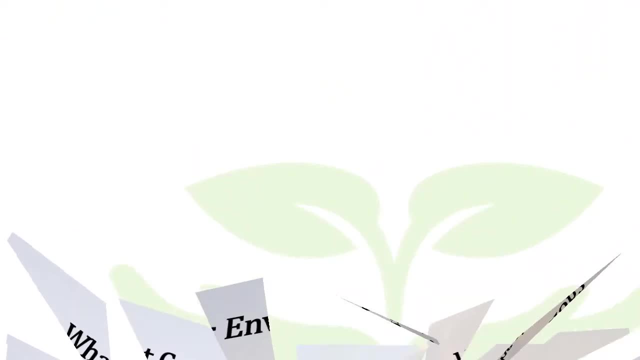 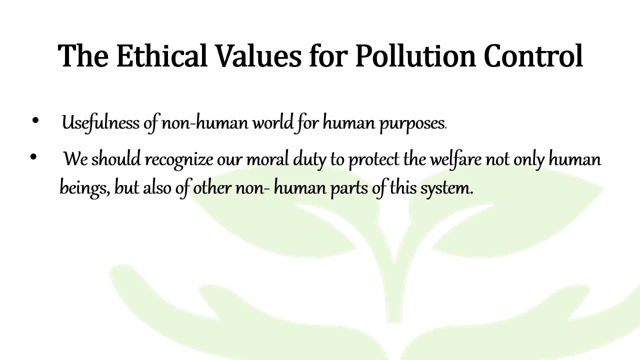 the near future. I hope you get it. The ethical values for pollution control. First, usefulness of non-human world for human purposes. Do you know the deep ecology? The importance of deep ecology is they give us a strong importance to the preservation of. 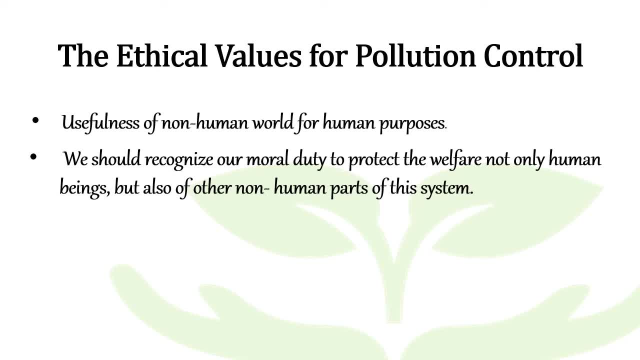 the global natural equilibrium, the variety and complexity of living beings, ecosystem and cultures. Second, we should recognize our moral duty to preserve the environment. We should recognize our moral duty to preserve the environment. We should recognize our moral duty to protect the welfare not only human beings but also. 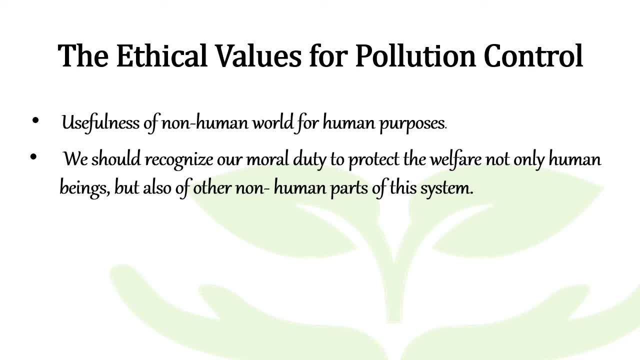 of other non-human parts of this system. Therefore, human beings have a moral obligation to conserve the environment in order to make a certain our survival and the survival of other species. Other than this perception, some people are caught up in their own self-interest. 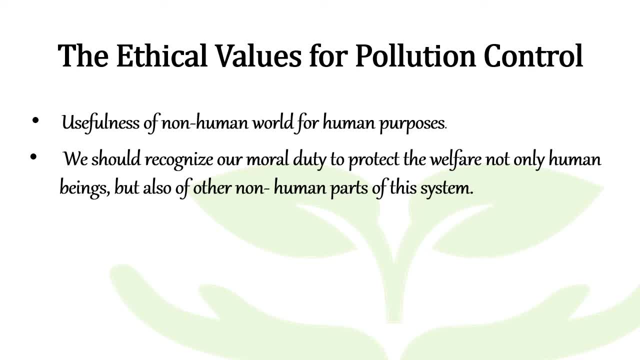 deviating from their moral obligation of environmental protection. Third, humans have no rights to reduce this richness and diversity expect to satisfy vital needs To deep ecologists. the mainstream of environmental groups' viewpoint of working to protect only those parcels of nature that are useful or necessary to human is a shallow ecology. 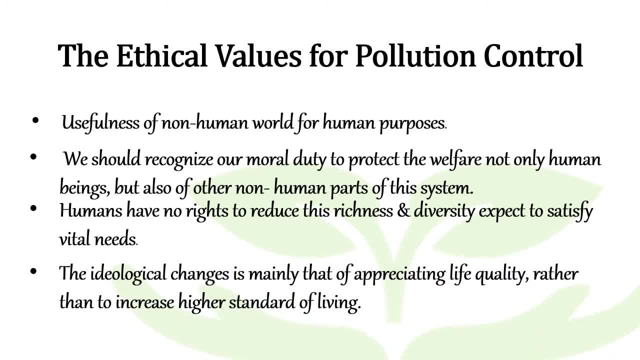 The last one is the ideological changes is mainly the appreciating life quality of the people, rather than to increase higher standard of living. According to deep ecology, the ideological changes is mainly the appreciating life quality rather than adhering to an increasingly higher standard of living. There will be a profound awareness of the difference between big and 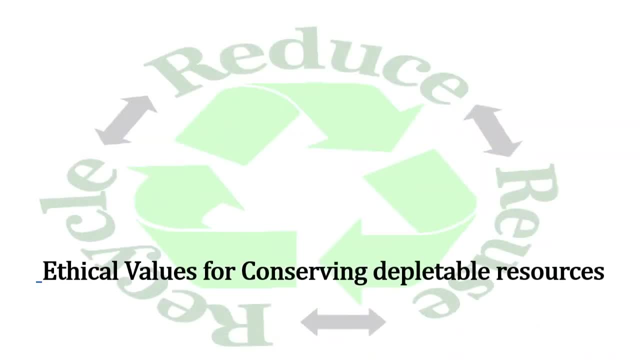 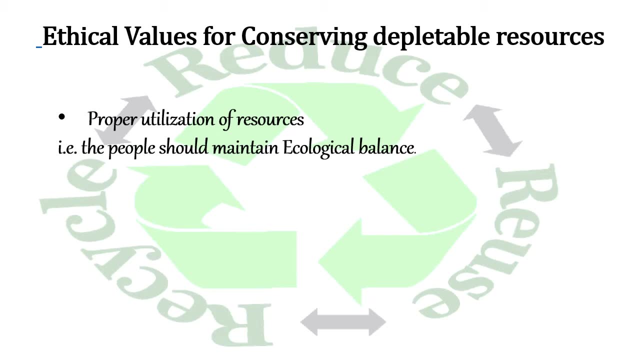 great Ethical values for conserving depletable resources. Proper utilization of resources. The proper utilization of resources is important for maintaining productivity because it prevents staff from underperforming or being overburdened by workloads or burning out. Projects can be managed with visible visibility, Reducing the risk of oversights. 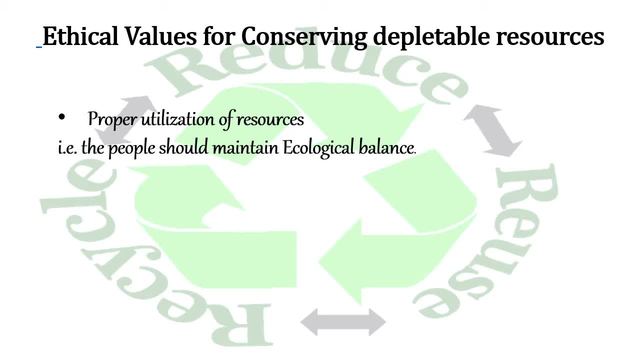 Using resources to their maximum potential gives you a better outcome. Second, we should adopt voluntary measures to conserve the resources. Getting involved in voluntary work has benefits that can last a lifetime, not only for those who you are helping, but for you as well. 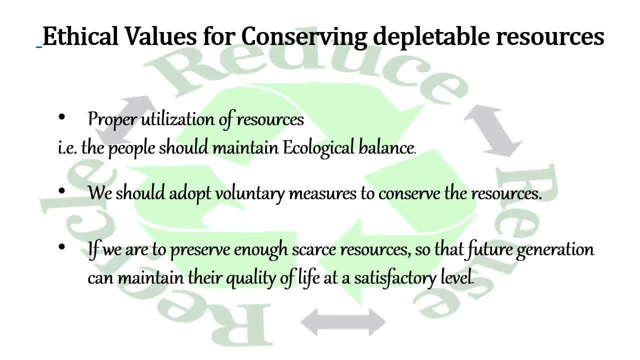 And lastly, if we are to preserve enough scarce resources so that the future generation can maintain their quality of life at a satisfactory level. Scarce reverses are, for example, are the workers, the equipment, raw materials, organized resources, equipment, equipment. 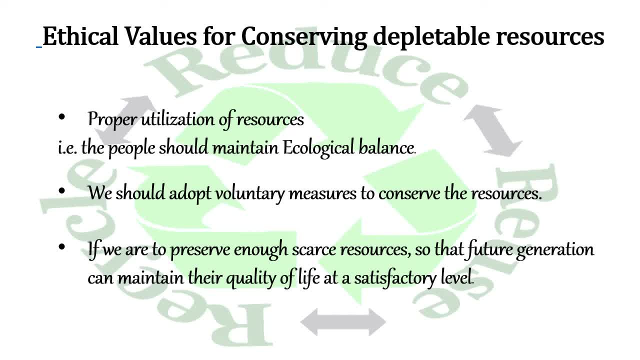 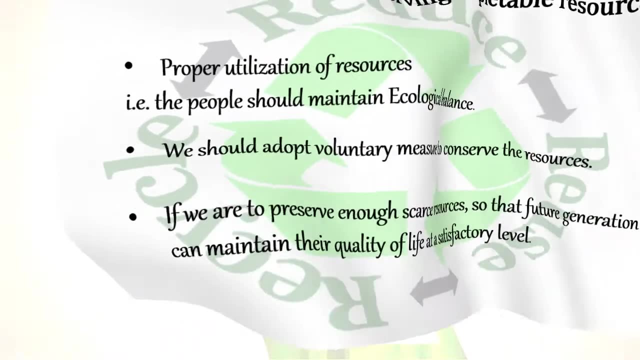 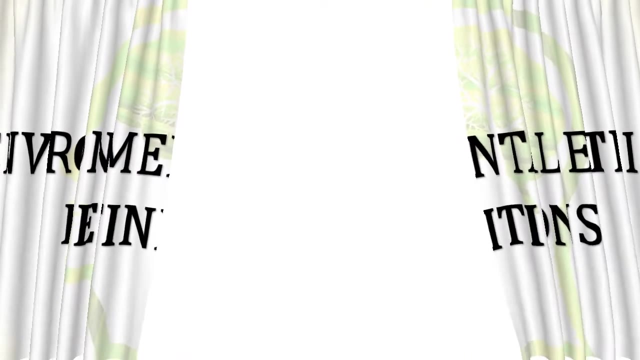 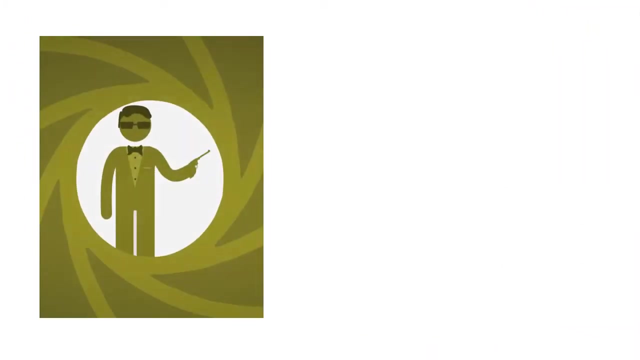 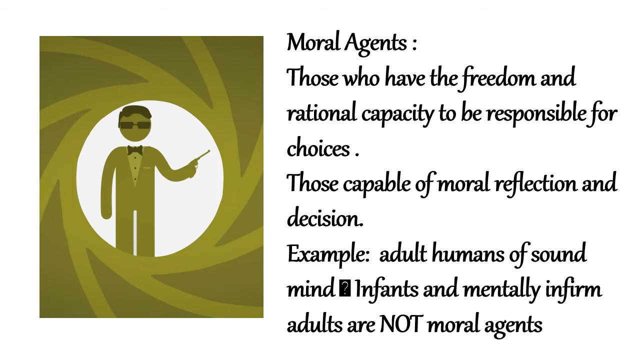 equipment, etc. Like more general society-wide condition of scarcity, a given resources falls into the scarce category because it has a limited availability in combination with greater potential, unlimited productive uses. Environmental ethics definition: Okay, Okay, The first one is moral agents. In short, we all care. 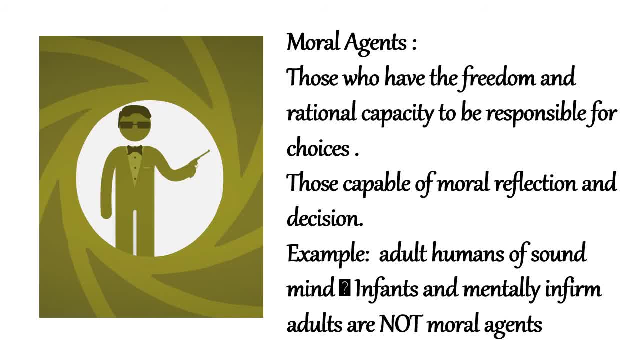 about. moral agent is simply a person who has the ability to discern right from wrong and be held accountable for his or her own action. What he does have a moral responsibility, of course, not to cause unjustified. them are just the five harm. Traditionally, moral agents are not responsible for the entrails of the 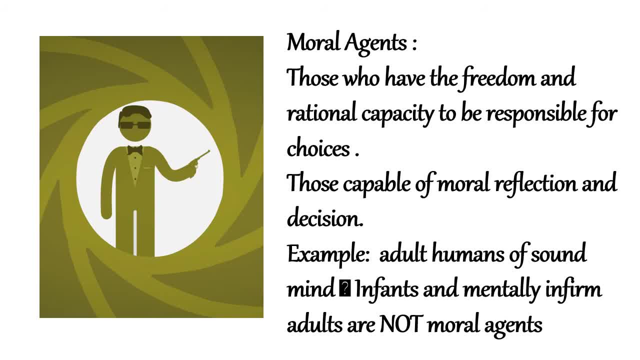 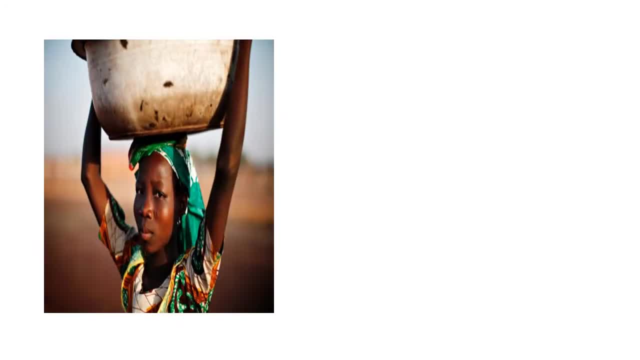 enemy's enemies. This is an inhumane act of an individual who is making resources for his Moral agency is assigned only to those who can be held responsible for their actions. Second one is moral standing. Simply moral standing. it is like your status, your condition. 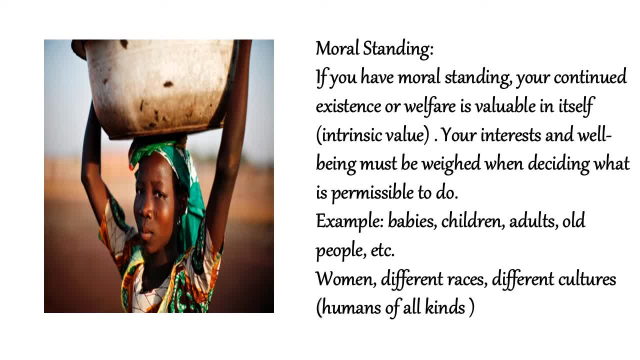 In ethics the status of an entity by virtue of which it is deserving of consideration in moral decision making. Moral standing is often key to open topics in debates like animal rights, bioethics, medical ethics, environmental ethics, of course, Because all have rights. 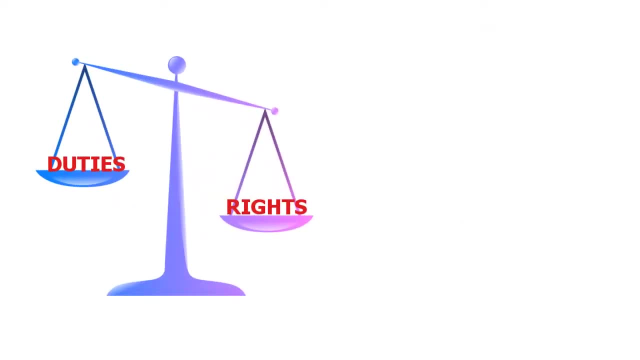 And lastly, is moral obligation. Moral obligation, it is also synonyms to moral duties, A duties which one owes and which he ought to perform, But which he is not legally bound to fulfill. These obligations are of two kinds. First, those founded on the natural right as the obligation to be charitable. 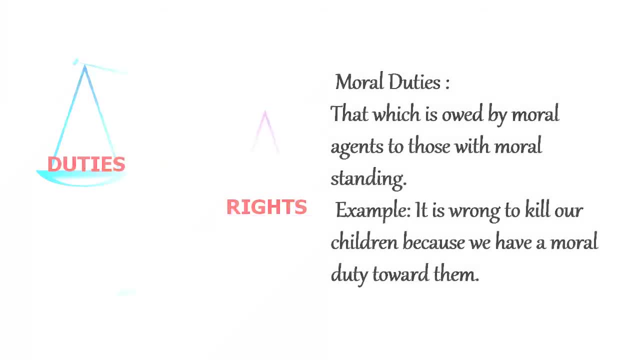 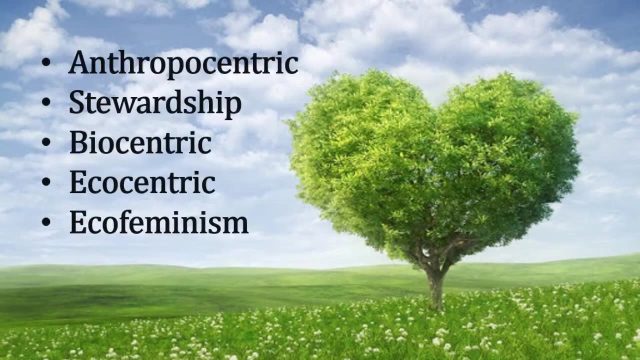 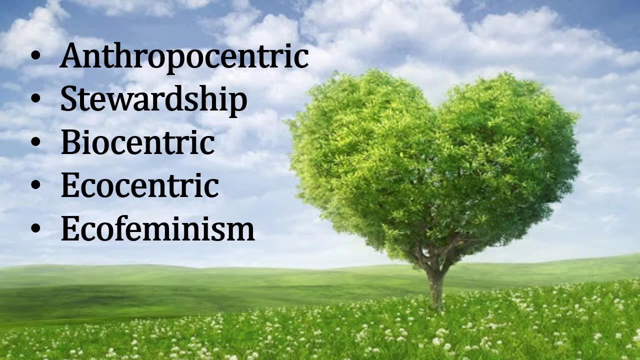 Which can never be enforced by the law. Now let's move on from various worldviews and ethical perspectives. These are anthropocentric, stewardship, biocentric, ecocentric and ecofeminist. You need to remember these. 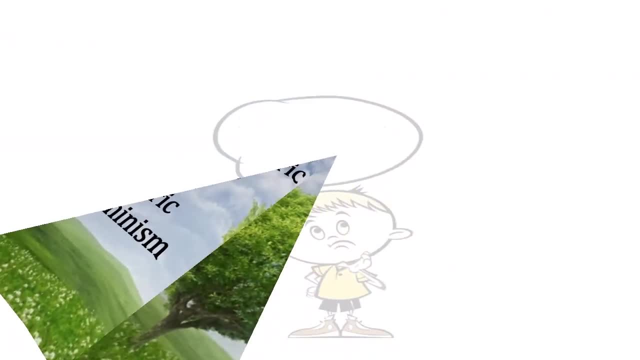 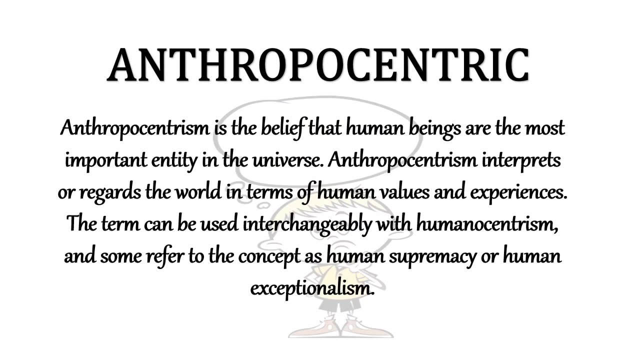 These are important First. okay, First is anthropocentric, Basically anthropocentric. it is just a like human. Humankind is the most important element of existence, Especially opposed to God or animals Like Bida. 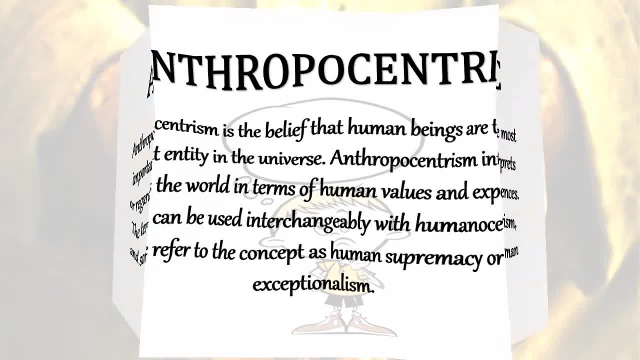 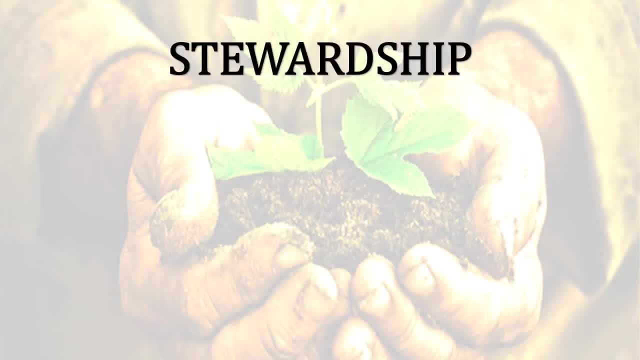 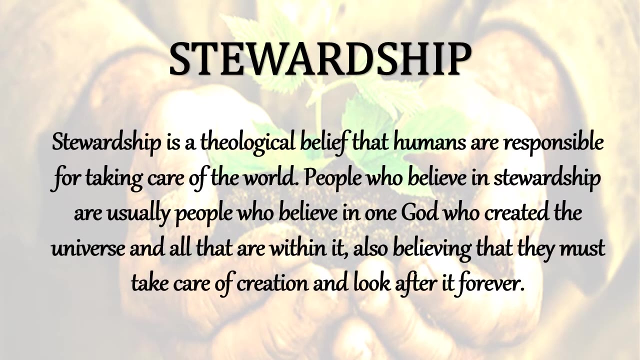 People are called bida. That's the focus. Next is stewardship. These are the people who are banal version. Stewardship is taking care of something like a large household. It is like a biblical worldview of stewardship. It can be consciously defined as utilizing and managing all resources God provides for all the glory of God and betterment for His creation. 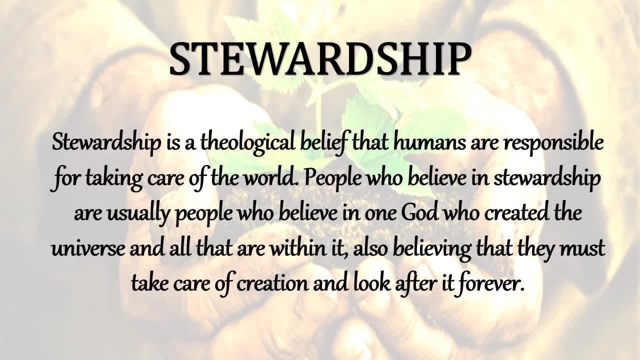 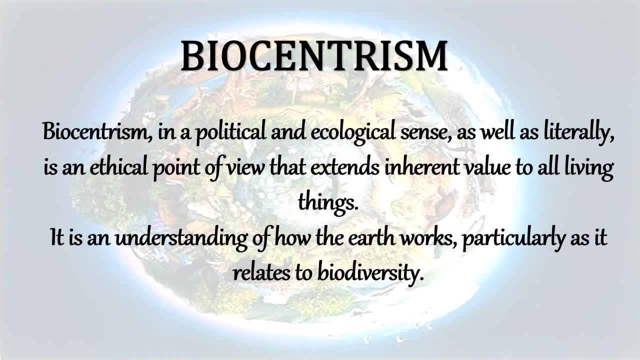 Right, Those are the good ones. That's the view. Next one is biocentrism. This one, in short, It is the view or belief that the rights and needs of humans are not more important than those other living things. These are the people who are not independent. 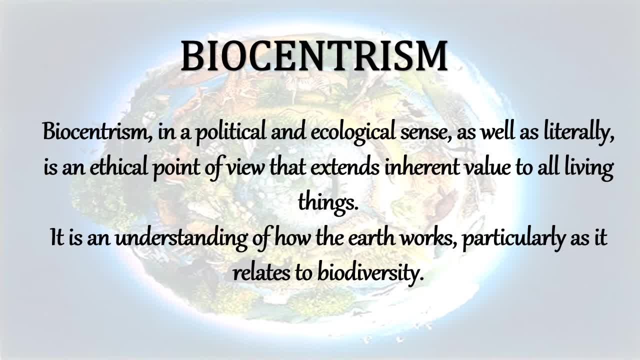 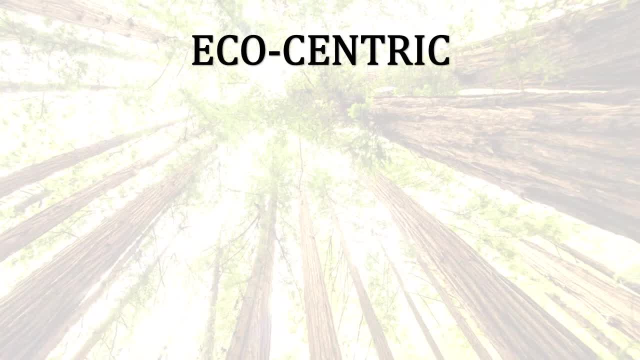 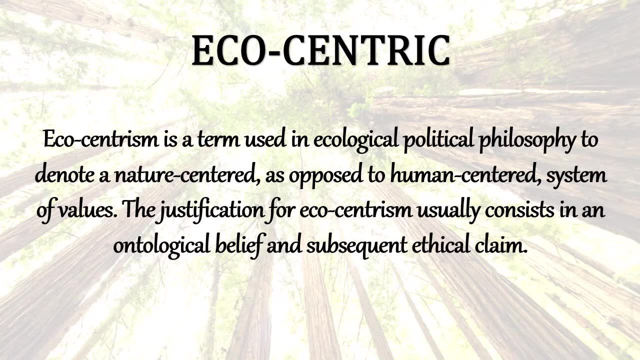 They are selfless. This is their view. They are biocentrism. Next one is ecocentric And ecocentrism. how do I say this? Example: strip mining, For example. strip mining, it harms the environment. 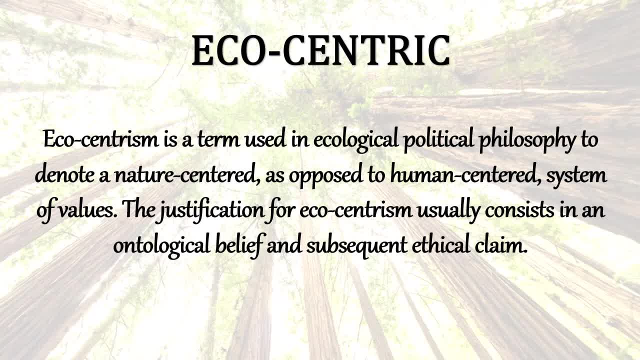 But it can also make natural resources that are available to us For the humans that we need to survive. So ecocentrists, people with this view, would argue that because this is so harmful to the environment, As long as it affects nature, it is immoral for them. 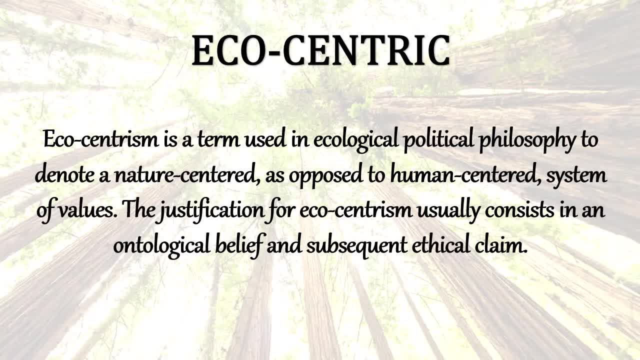 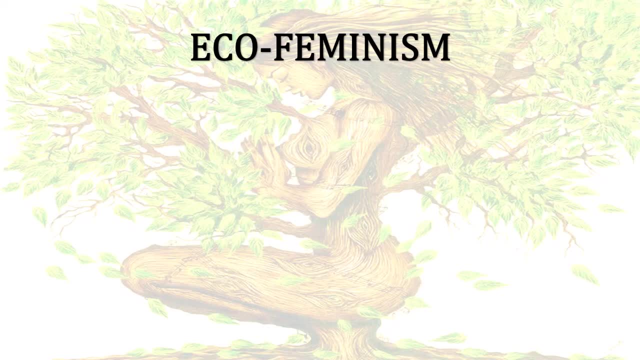 So therefore, environmentalist policies are generally ecocentric in nature, Often Environmentalist. As long as it harms nature, it is immoral. They are like that. Lastly, is ecofeminism- There is a clue- Feminine. 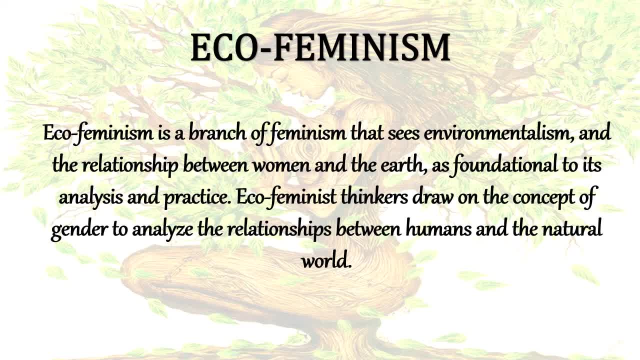 Women. It is a branch of feminism that is related to the environment. It is like a relationship between women and earth. It is like that. It is like a foundation. People like this- Most of them, are women Like us- Oh my God. 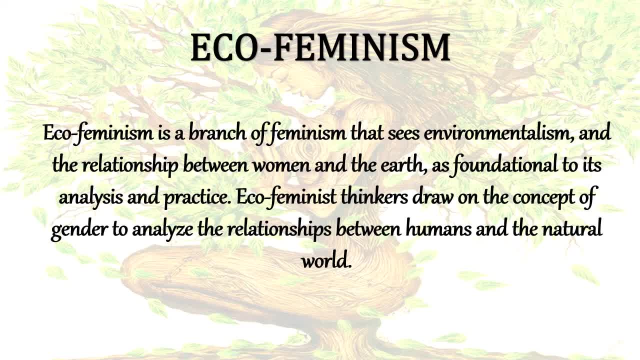 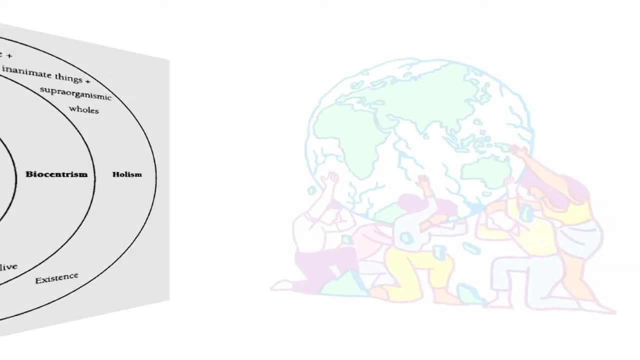 They are called ecofeminists. Ecofeminist thinkers draw a concept of gender to analyze the relationship between humans and natural world. That's it, Okay. That's all So that you can do it better. And The following short video is about protecting our planet and combating climate change.